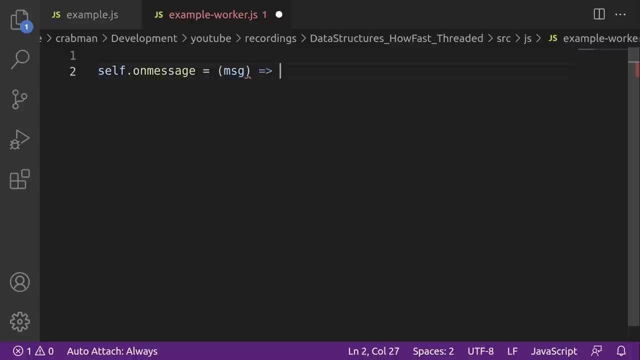 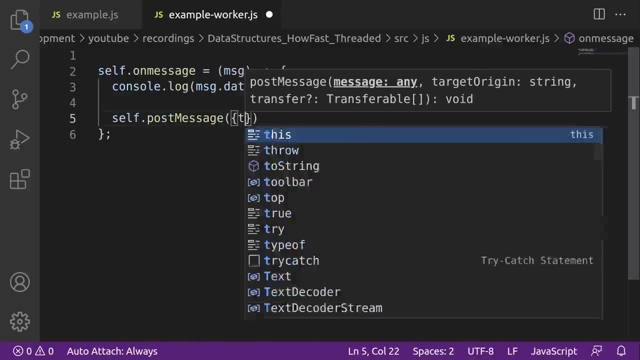 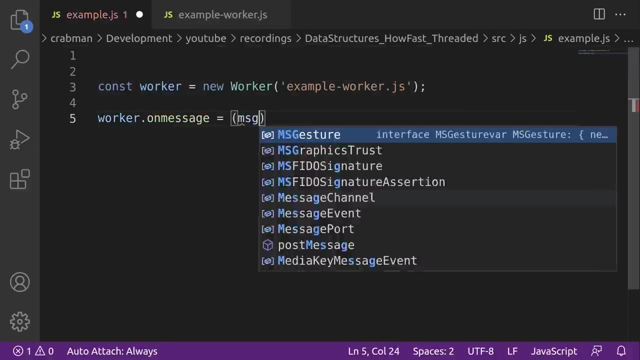 and the code that runs in here will actually be running in another thread, off the main thread, And we need to define an onMessageHandler in here, and for now we'll just have to run it in the main thread. Now in the main script I'll declare an onMessage for the worker object, which will just again: 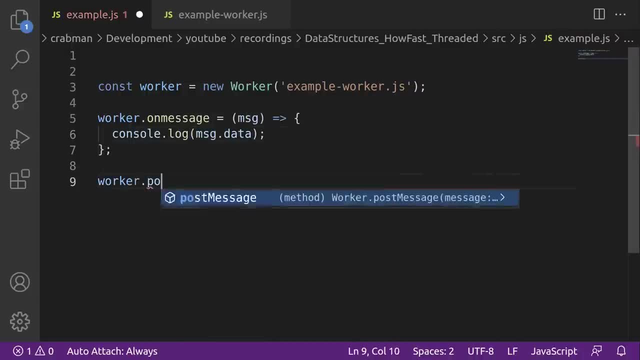 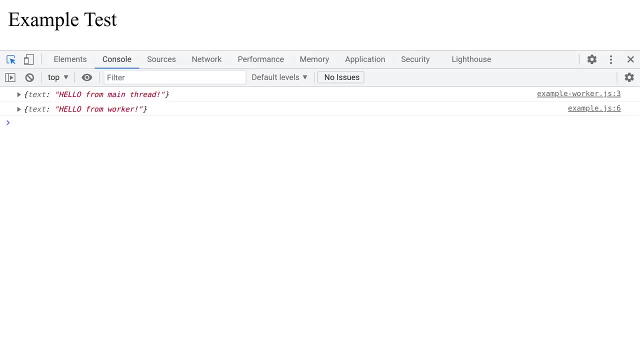 log some crap in the console. Then we can post a message to the worker using the postMessage function, and we should be good to go Running this. all you can see the log statements show up in sequence in the console and that's the gist of it. So let's speed something up using workers. 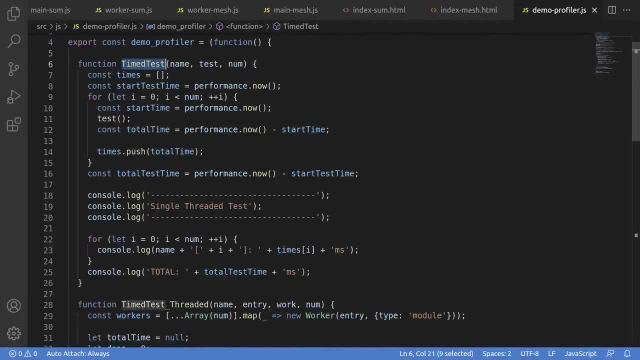 I've gone ahead and made this dinky little testing harness just to make things a bit easier for us. It'll just take a test, run it a bunch of times, recording times using performancenow. After all that, it'll spew the results into the console, both individual runs. 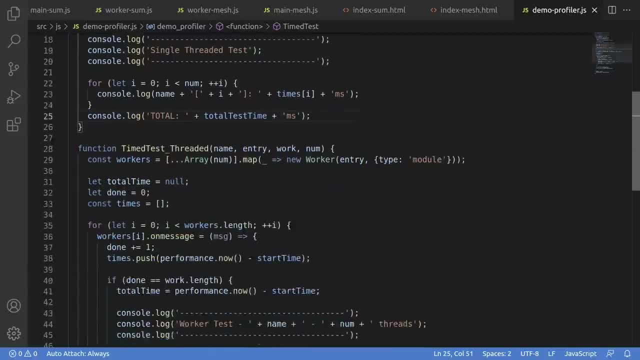 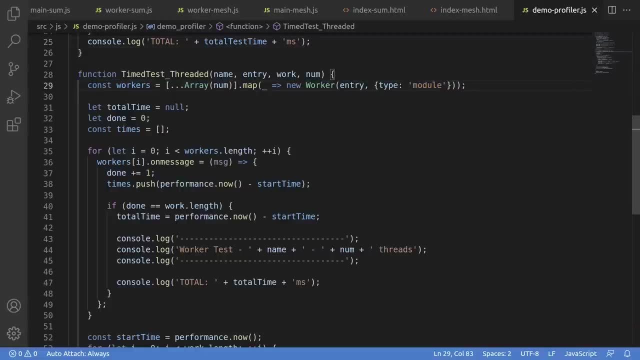 as well as the total accumulated time. There's a threaded version too, and that basically does the same thing, more or less. Specifically, we create an array of workers to start. Then we have a loop here which sets the onMessage. 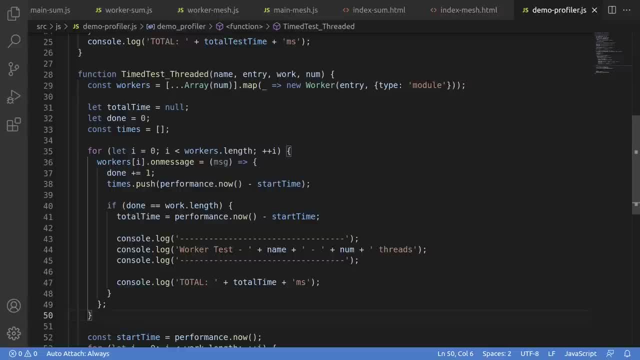 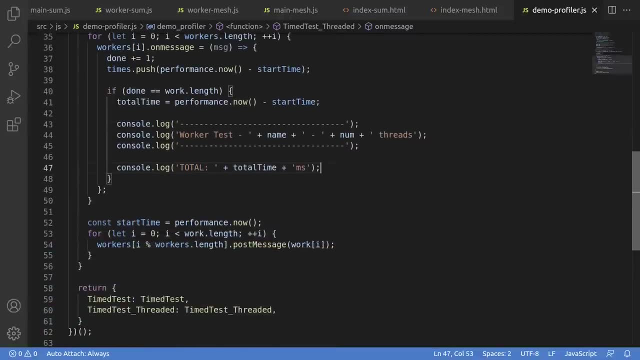 and this is where we can look to see if this is the final bit of work to be done. If it is great, Record the time since we started and throw that into the console. Finally, this last loop actually loops over the work items, doling them out to the workers. 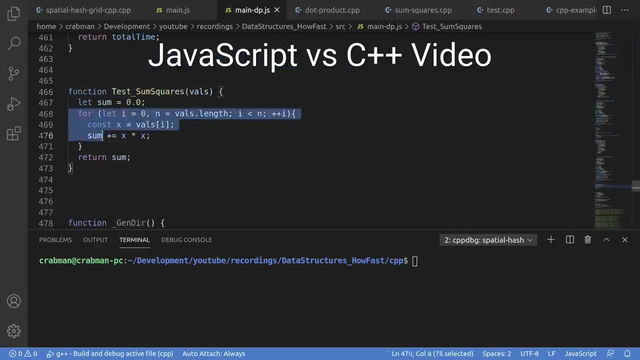 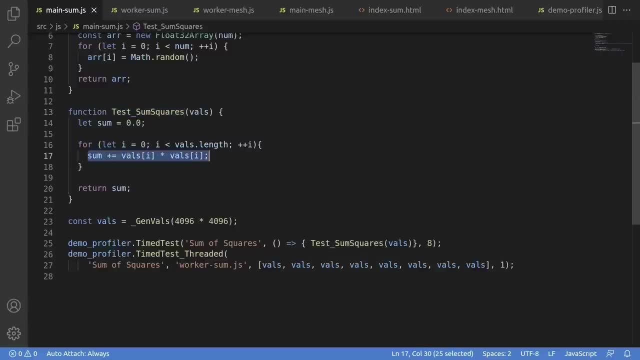 In the previous video we covered comparing C++ and JavaScript, so let's just go ahead and grab the first test we did there, the sum of squares. Recall that this test really just generates a bunch of crap data in an array, then loops over it, doing some pretty much pointless math. 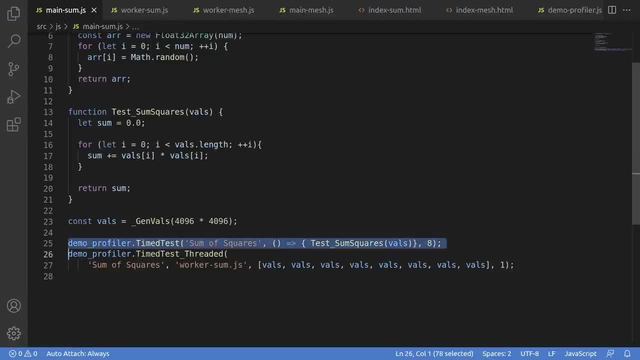 squaring the values and summing it all up. To start, the first thing that runs is the single-threaded version, and we'll do the test a bunch of times. In this case I just did the test eight times and that'll just kind of be the baseline to compare to. Afterwards. we can go ahead and 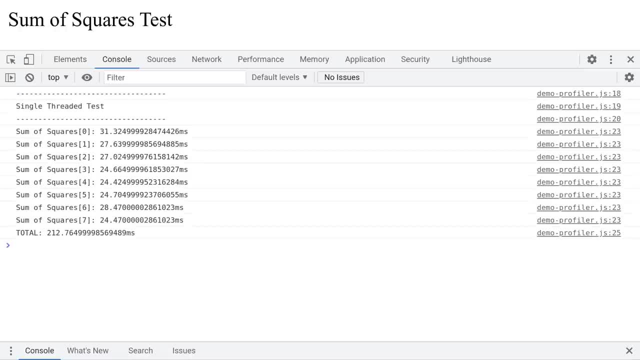 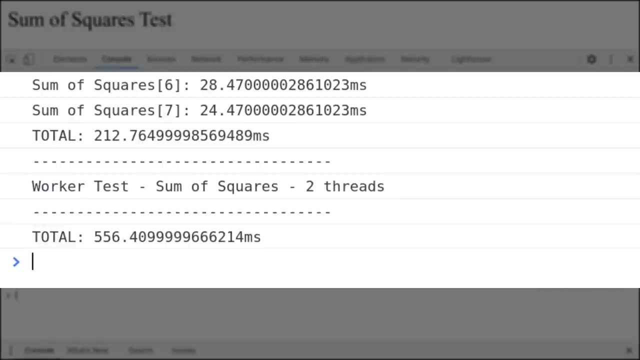 run the threaded version, and I'll do that on two threads. to start, Your first thought might be: with two threads we'll go twice as fast, But the first thing you notice is this actually ran slower than the single-threaded version. So what gives here Shouldn't have. 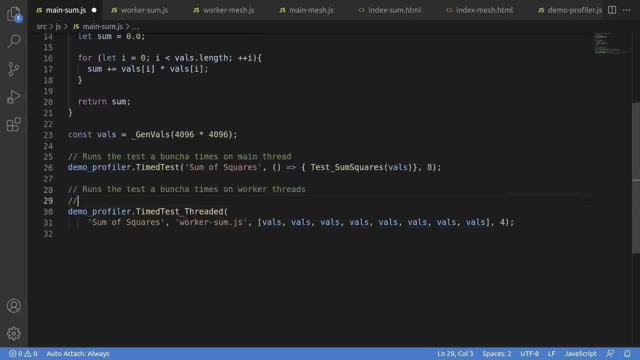 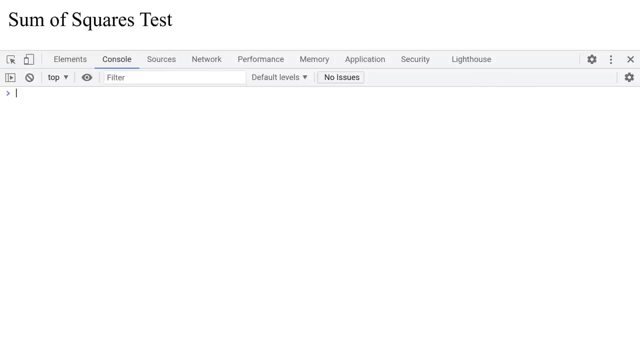 this been faster. We can try screwing around with the settings a bit more, see if that helps. So if I bump this up to four threads, we see some improvements. I can keep jacking this value up six threads or eight threads, But we're kind of seeing a pattern emerge here. The improvements: 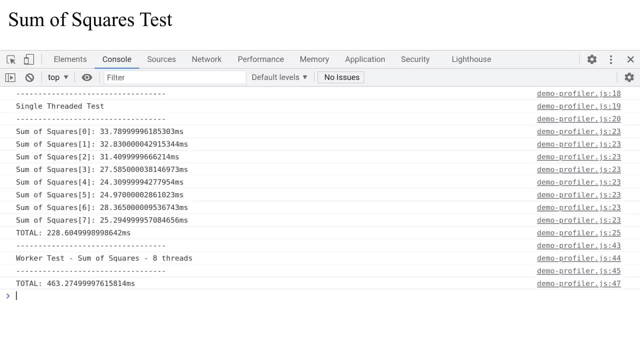 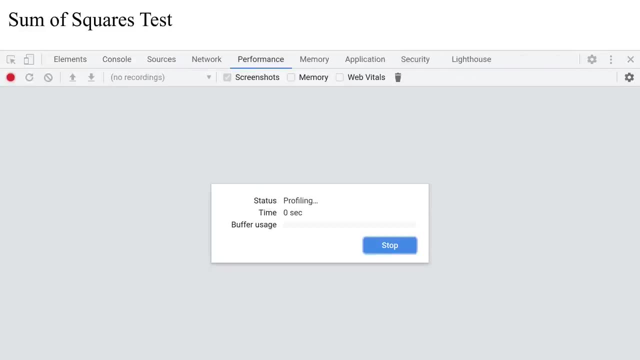 all kind of suck. I mean, they suck less and less as you throw more cores at the problem. but these were all outperformed by just doing it all on the main thread. Let's use the performance tab to analyze this a bit more closely. 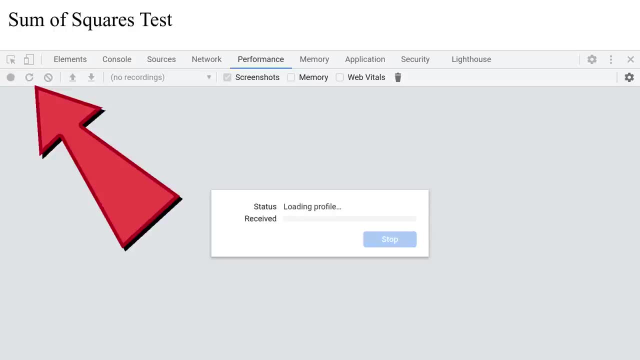 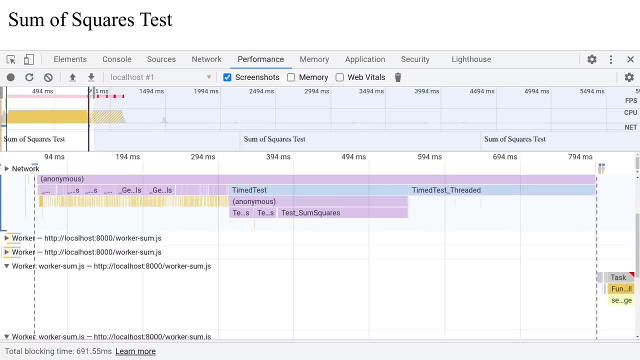 So I've used the reload and record functionality and it grabbed a couple seconds of profiling data. You can look at the main thread here. You can see all the individual calls to test some squares here. They all just kind of happen one after the other. Nothing really special to note. 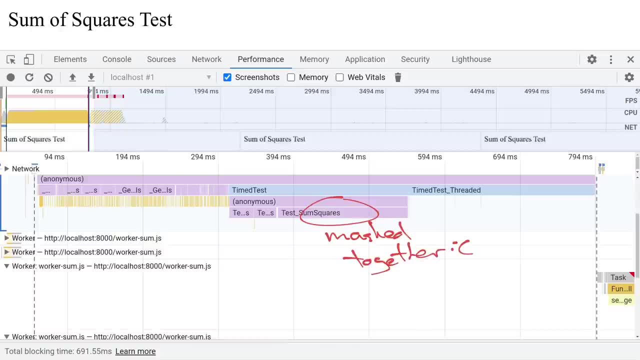 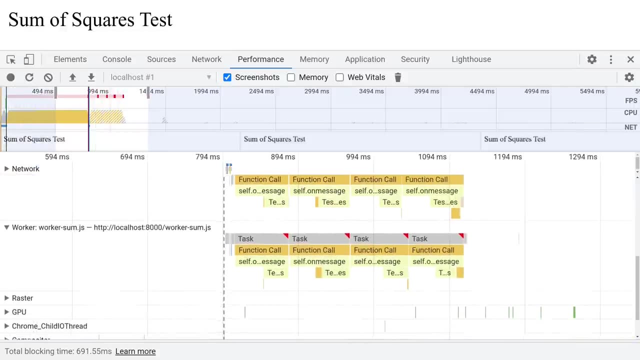 other than often. it seems to show the first few and then mashes the rest together, But you can make out that the timings are roughly 30 milliseconds per iteration Over here. this is the threaded test and from here we can scroll down and find the worker threads. 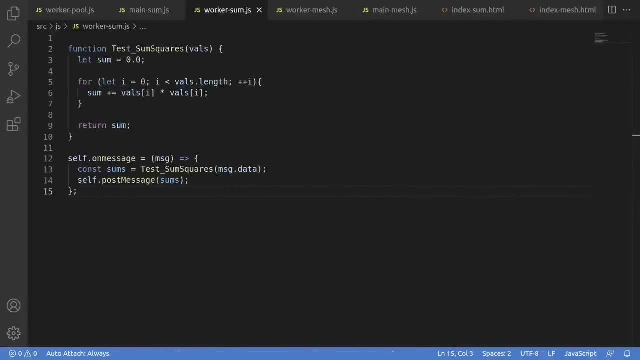 Notice how each of these work on message calls. We can bring up the code quickly, but there's almost nothing in here. We receive the data from the main thread, run the benchmark and then post it back And from the profile. these on-message calls take considerably longer than the main thread. 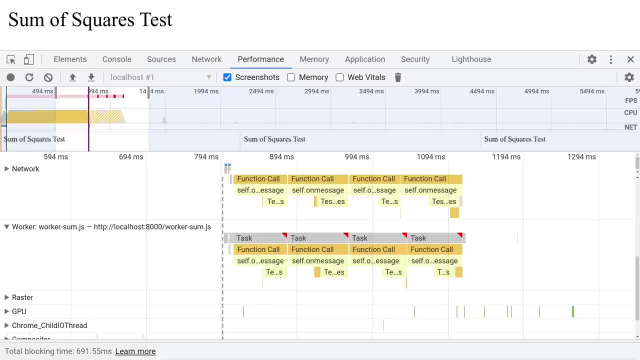 benchmark runs. We're losing a ton of time here. Notice how the test time only takes about 30 milliseconds or so on the worker, But the whole on-message call seems to take a lot of time And it's in the receiving and then sending the data that we seem to be. 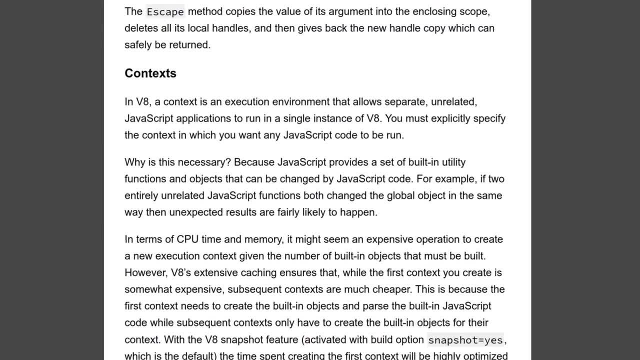 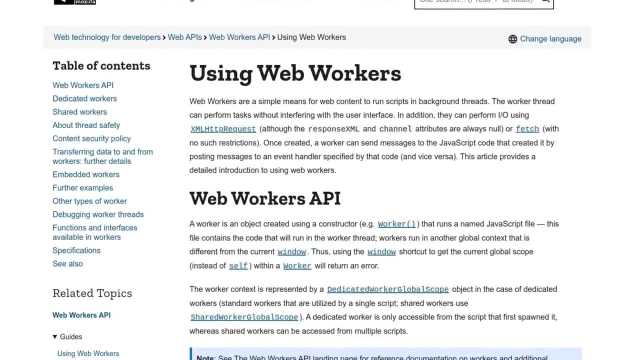 losing an enormous amount of time. Remember that each of these workers, in the same execution context that the main thread does. In fact, the MDN docs for web workers specifically state that data passed between the main page and workers is copied, not shared. 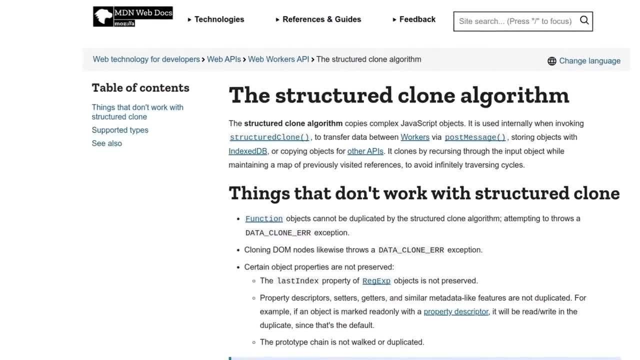 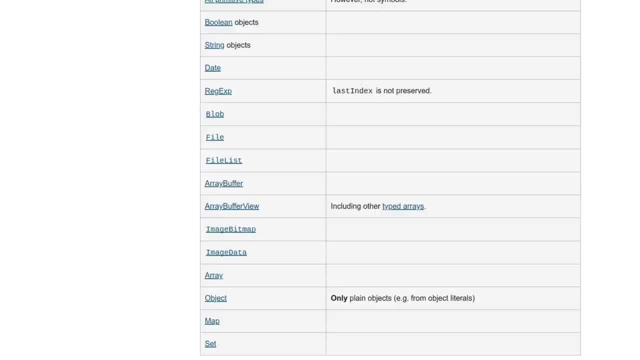 And that happens using the structured clone algorithm. We're not really digging into how it works, but intuitively copying data is never free, Although the closer and closer you get to a pure memcopy or just passing a pointer, the faster the copying is. 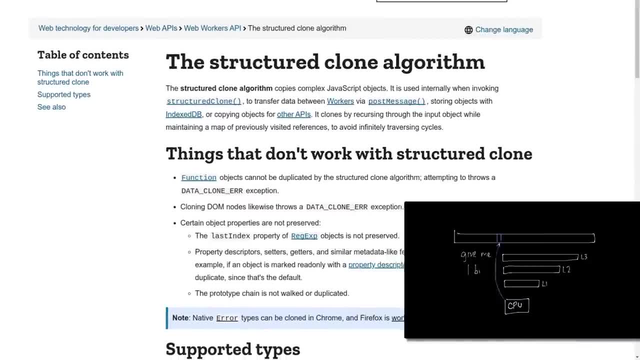 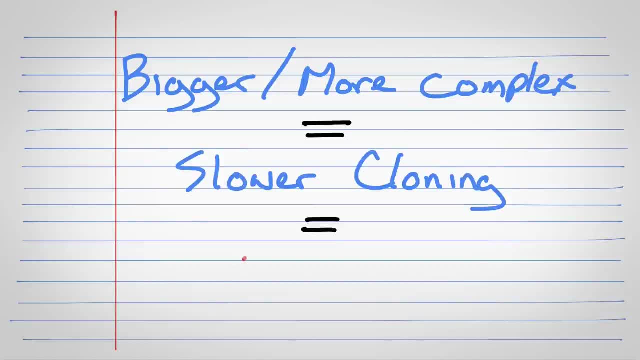 Just watch the video on CPU caches if that doesn't make sense to you. So you can intuitively believe that the more complex the data, the slower the structured clone algorithm will be and thus the slower post-message will go. And luckily I didn't have to actually confirm that myself. I found this website from Surma. 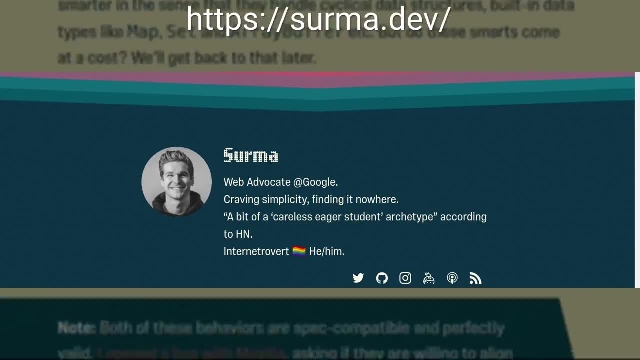 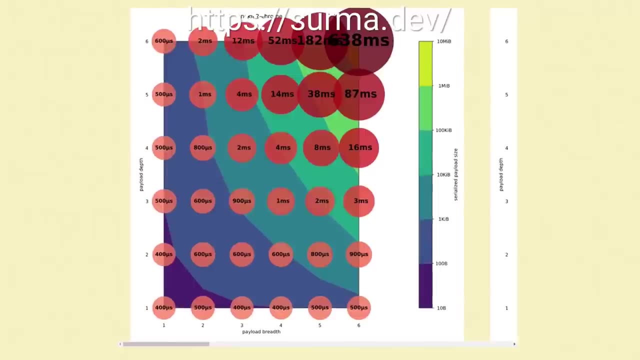 a web advocate at Google, and they looked into the cost of post-message. so I don't have to, I can just point out their work, And what they found was the larger and more complex the objects you're copying, the slower things go, To the surprise of. 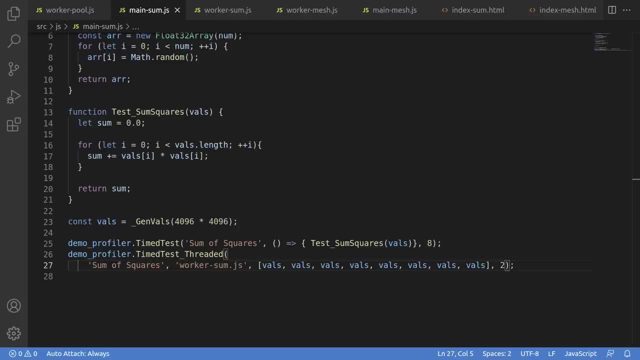 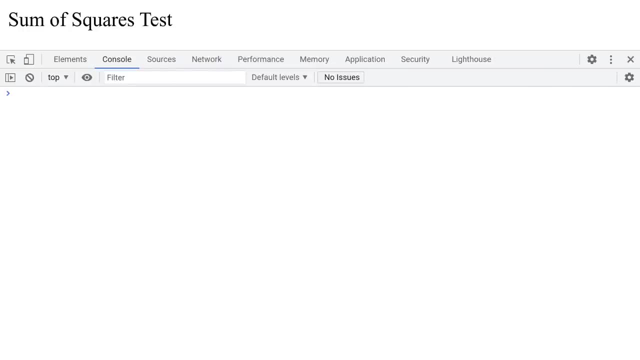 absolutely nobody, But it's good to confirm it And to just hammer the point home because I have nothing better to do. we reduced this test to one thread and, surprise, surprise, the performance of the threaded version absolutely blew, because we're doing just about everything wrong. 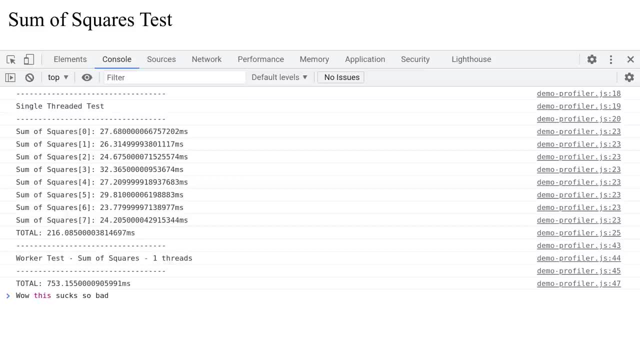 The takeaway here is that to go faster in a threaded environment requires a bit more finesse and planning than just throwing crap at another core and thinking it'll all work out. So let's examine a more realistic situation where we'll make things go faster. 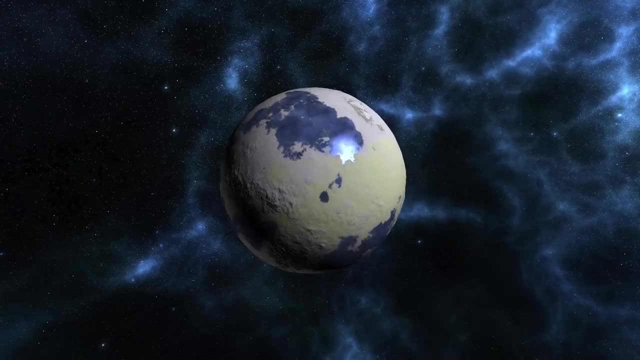 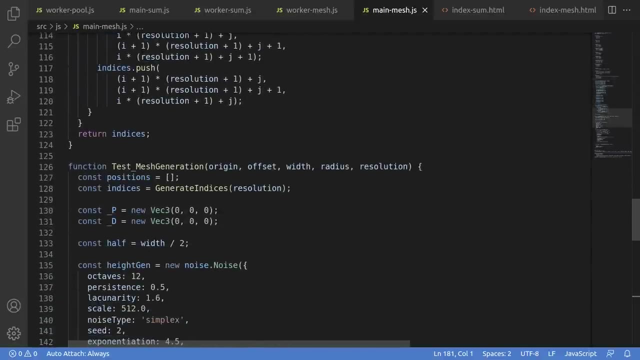 For a while I've been doing a series on building procedural terrain and we do a lot of the mesh building in separate threads. The nice thing about this test is that you're mostly just sending a few simple parameters there. that takes almost zero time to serialize. 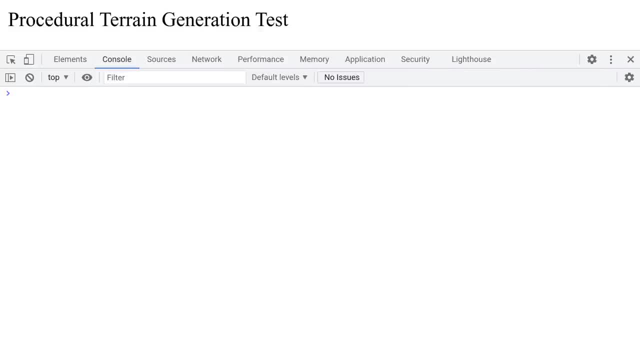 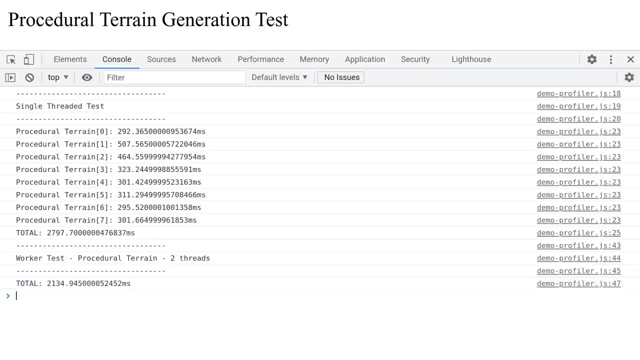 and all the work is procedurally generated. So we can run this the first time using two threads, and what you see right out of the gates is a gain for the threaded version. It's quite a bit faster- Not twice as fast, considerably faster, So we'll take the win. 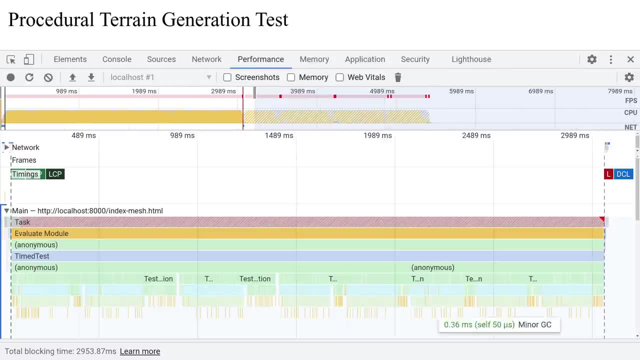 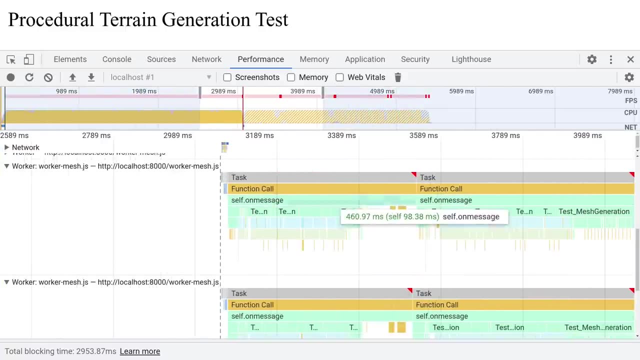 Let's take a closer look using the performance tab again. So what I've done is recorded a profile and we can poke around a bit in here. Look at these on-message calls. What you notice is that the tasks seemingly start right away. 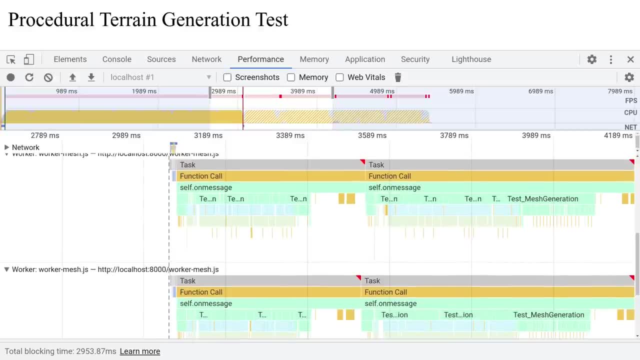 which kinda jives with our expectation, since the deserialization cost now should be really small, since we're sending so little data to the worker. But the worker generates the mesh data and has to send it back, and that's still costing us quite a bit of time. We can trivially confirm that it's. 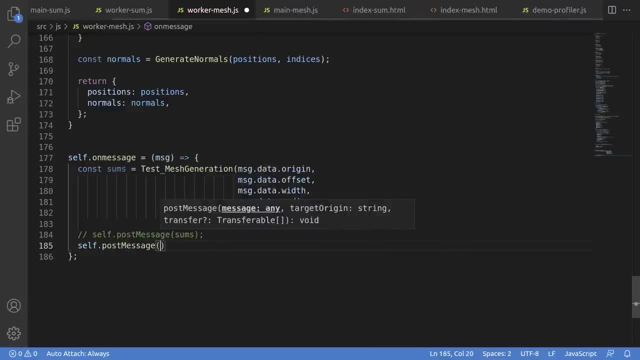 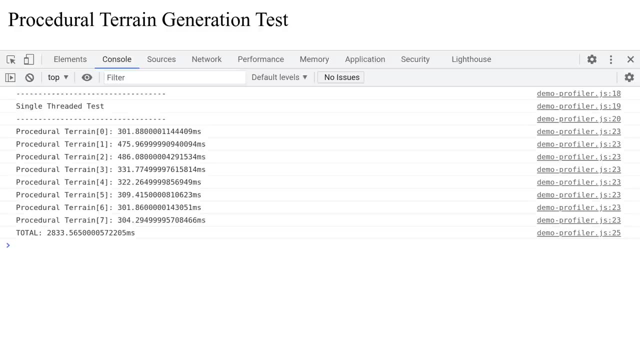 time by sending back a dummy. dict V8 isn't smart enough to optimize that work out, so this will force us to actually build the mesh, but then throw that work away and send back nothing, And what you'll notice from the results is that we're getting a lot closer to the 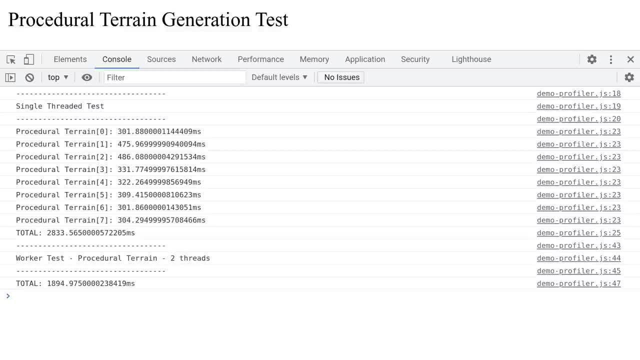 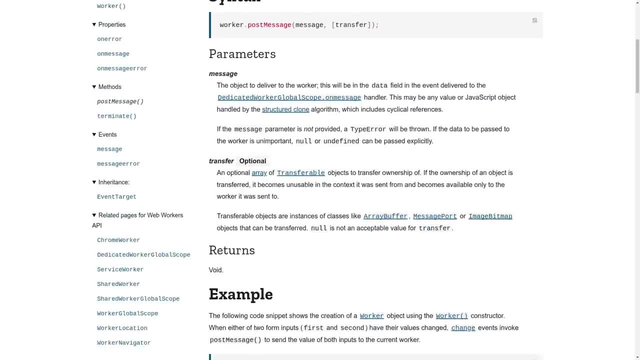 performance being twice as fast being on the workers. So that tells us that we need to kill that serialization cost. The MDN docs show that the post message function takes two parameters: The message which is transferred via the structured cloning, and then this transfer. 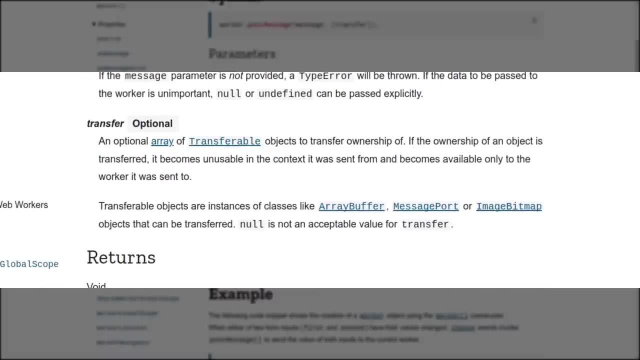 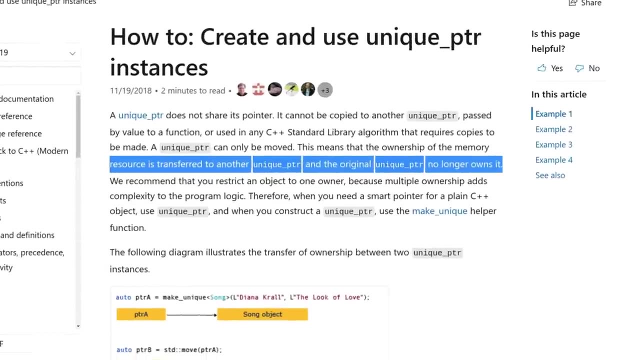 argument. which is more interesting, This lets us transfer the ownership from one execution context to another, Or in other words, this is a lot like moving a unique pointer in C++, And the upside is that you don't have to copy all that crap over. So this is potentially awesome. 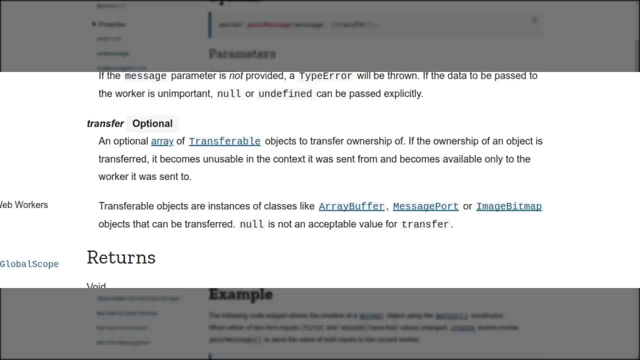 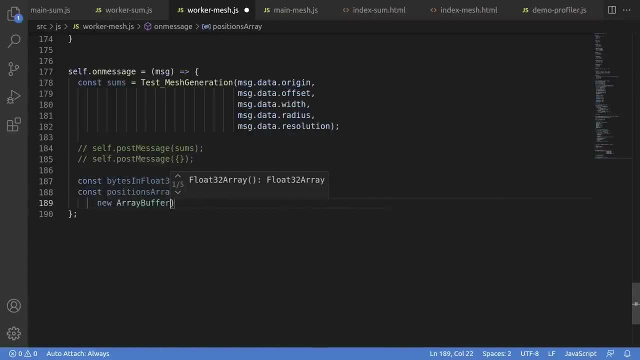 The only small caveat is that it has to be one of these specific types that implements the transferable interface like array buffer In the code. here, instead of passing the results directly to the message parameter, we're going to pass the error to the target and it's going to pass the error directly to the message parameter. We're going to pass the error to the target and the error will transfer to the code and it's going to pass the error directly to the message parameter. We're going to pass pack everything into a couple of array buffers. 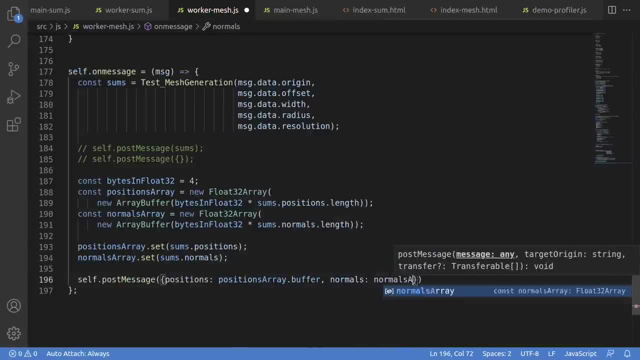 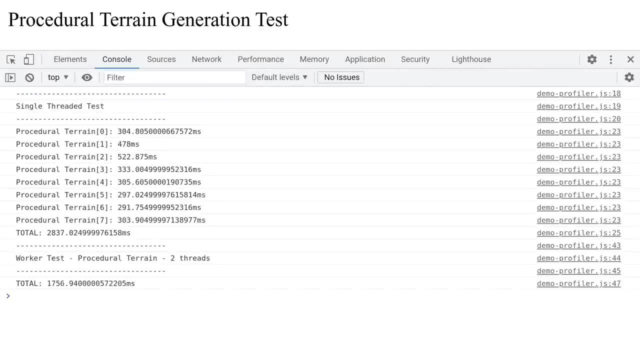 So this block of code just allocates them in some float32 views, packs everything together and then posts it and sets the transfer arguments. Now we run this and, yay, it's actually really close to the same speed as passing absolutely nothing back. 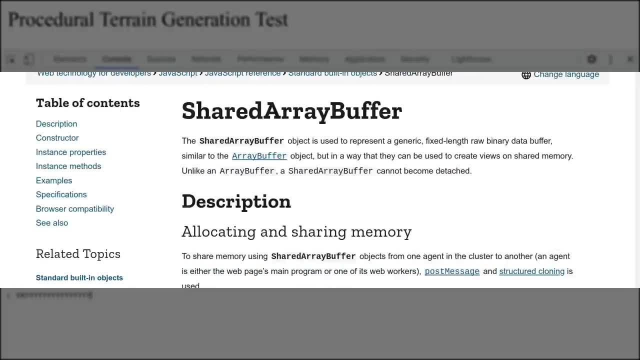 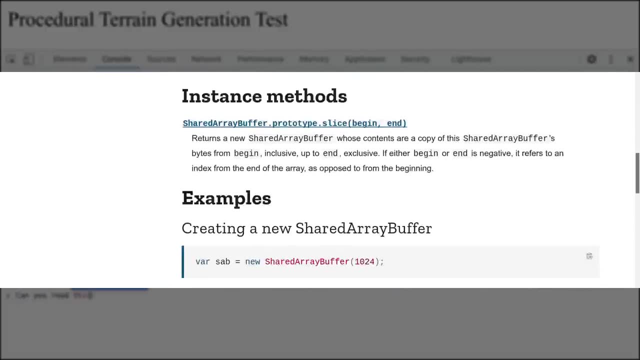 So this is a big win. Quick little aside note: you can also pass shared array buffers back and forth between workers in the main thread and even read and write simultaneously from the same buffer from multiple threads. Just remember that you need to use atomic operations to mitigate against concurrency. 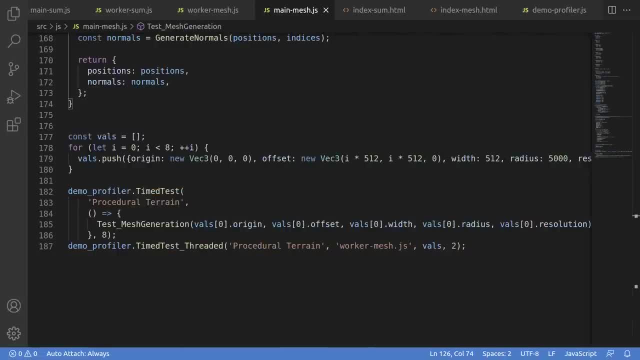 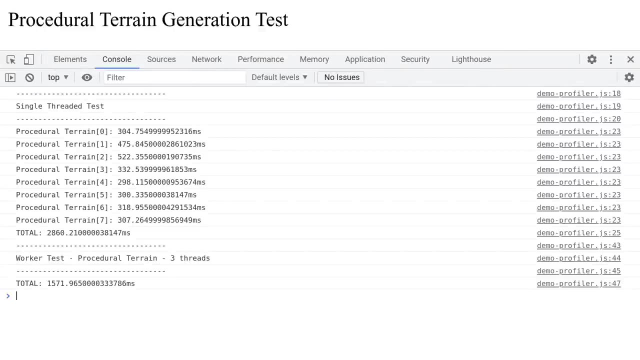 issues. We can talk about that in another video. Anyway, that aside, now that we have a lot of the speed, let's start jacking up the threads. So with 3 threads we see a good improvement over the 2 thread case. 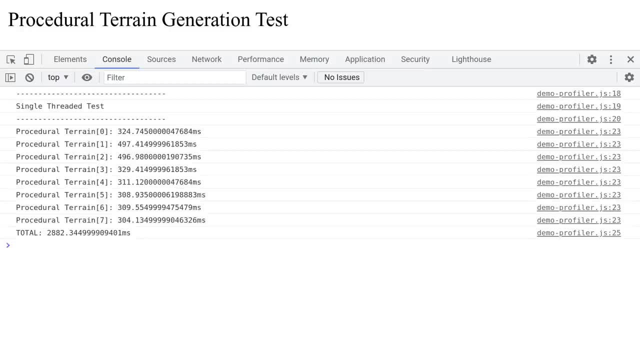 And another good jump at 4 threads. At 5 threads, though, we didn't see much, if any, gain, which is a little strange. I push this up to 6 threads and again nothing. At 7 threads, we're still seeing pretty much the same timings that we saw with 4 threads. 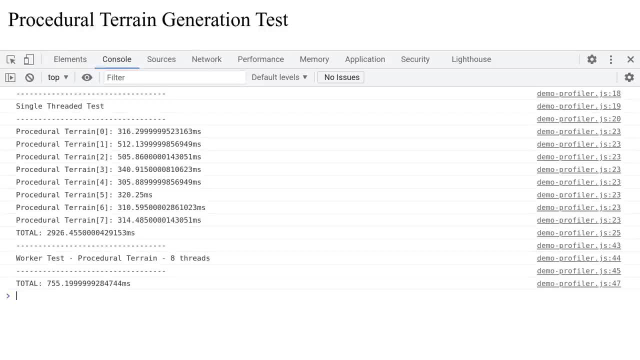 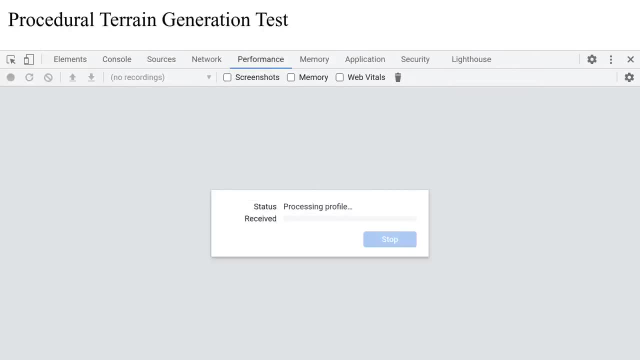 But when I bumped this up to 8 threads we suddenly jumped. This is really interesting. We kind of have a performance cliff here. Throwing more threads made zero difference until we hit 8.. Using the performance tab, we can take a quick profile and that reveals the culprit right. 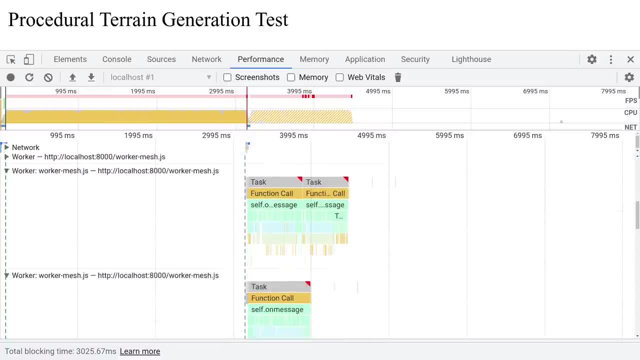 away. So from this you can see that this worker here is getting 2 sets of work And everyone else has to kind of just sit around twiddling the thumbs, since the amount of work wasn't divisible If we just jack up the number of work items and play with things. 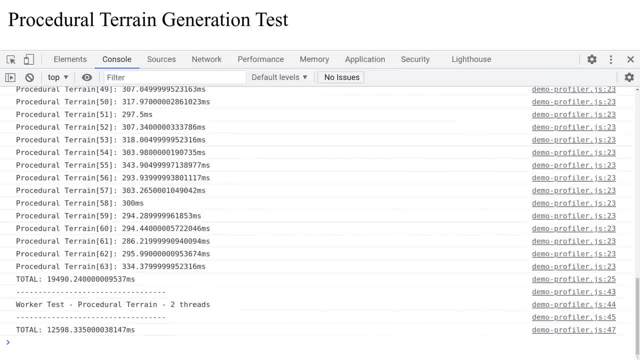 So let's just go with 64, doesn't really matter. And on the first run we see around 20 seconds or so give or take on the single threaded version, Versus 12, 12 and a half seconds for the 2 thread version. 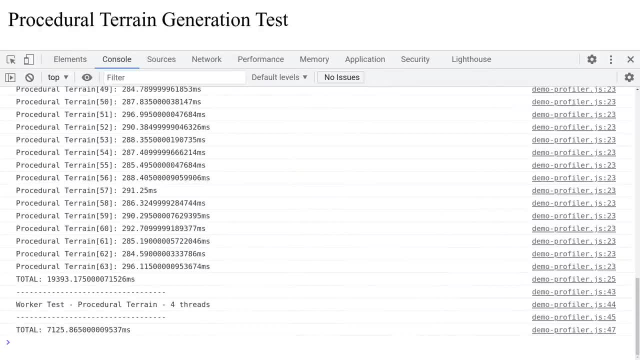 Fantastic improvement Almost twice as fast. At 4 threads we're still seeing good results around 7 to 8 seconds or so- Pretty great. At 6 threads, though, we're starting to see a serious drop off, Getting somewhere in the 6 and a half to 7 second range, which is a really modest gain. 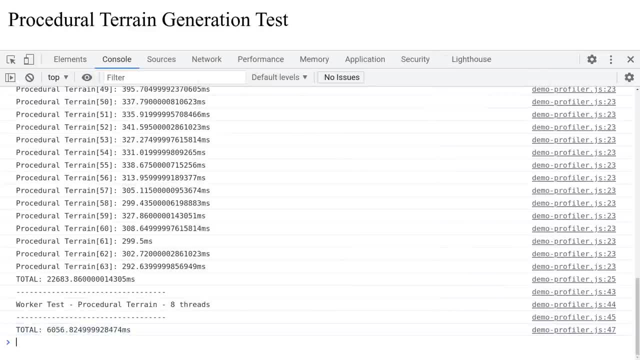 at this point At 8 threads. that only just barely nudges us further ahead. on top of that, I'm seeing low to mid 6 seconds, depending on the run. I tried running this at 10 threads and this ended up being slightly slower than the 8. 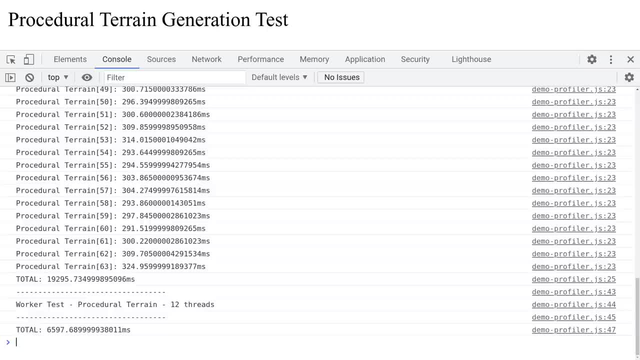 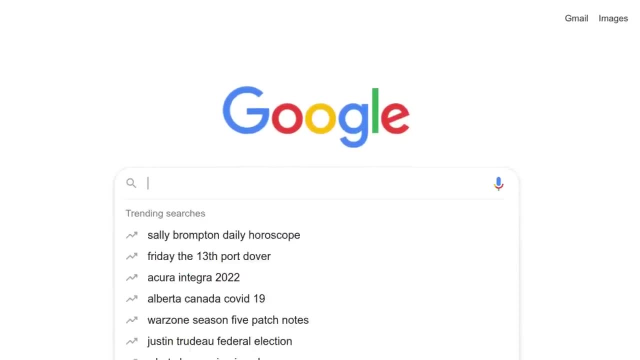 thread scenario, And at 12 threads. well, this is pretty clear that not only is this not getting faster, it's actually getting slower. So what gives? I don't have unlimited cores of my CPU and chances are you don't either. 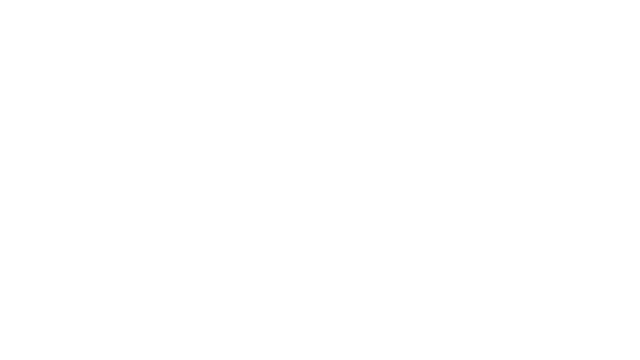 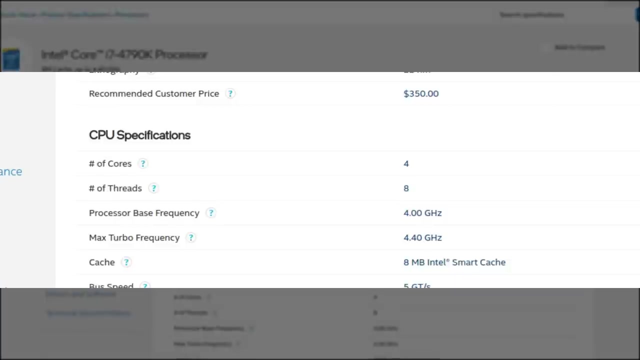 In fact I can look up my specific CPU. I have an i7-4790K. Some of you have said this is a pretty decent CPU, but whatever, it's an old one. Looking at the specs, you can see that it has 4 physical cores and with hyperthreading. 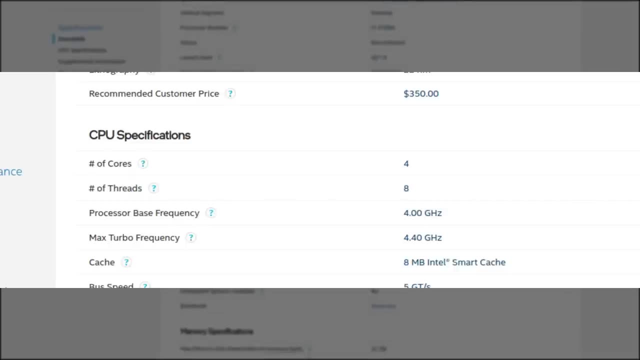 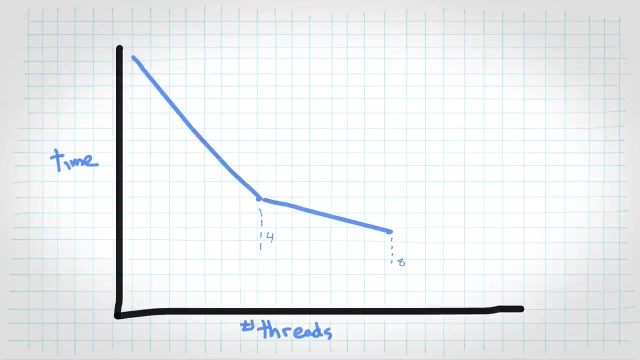 it has 8 threads And that correlates really well with our results: Strong improvements up until the 4 core mark and then really modest gains after that. I mean, we get gains, but after that we max out the hardware threads.